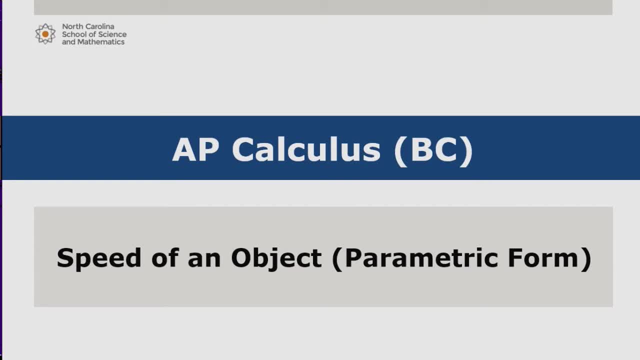 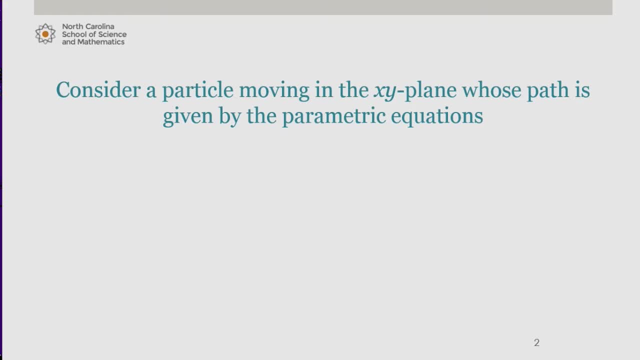 In this video we'll look at another example involving the speed of an object whose path is described parametrically. Consider a particle moving in the x-y plane whose path is given by the parametric equations: x equals t cubed minus 3t squared, and. y equals 2t cubed minus 3t squared minus 12t. 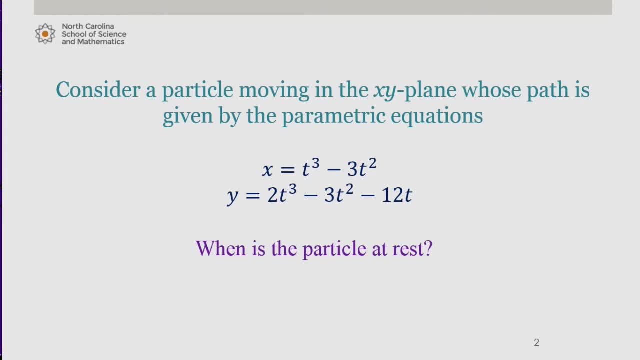 When is the particle at rest? Well, we know that the speed of the particle can be calculated by finding the square root of the sum of the squares of the derivatives of x and y respectively. So, in our case, with x being t cubed minus 3t squared plus 12t squared minus 12t squared, 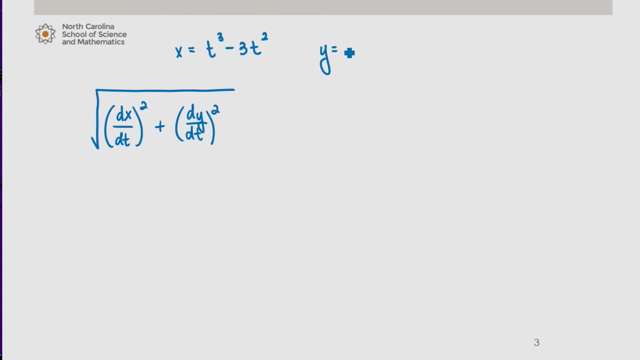 equal 12t squared minus 12t squared plus, into 2t squared minus 12t squared minus 12t squared squared, and y being 2t cubed minus 3t squared minus 12t. Our expression for speed is then the derivative. 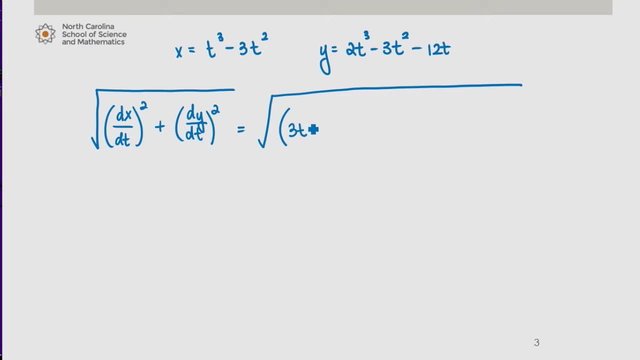 of x with respect to t, which is 3t squared minus 6t. We square that and add the derivative of y with respect to t squared as well. Now, since this is the expression for speed and we want to know when the particle is at rest. 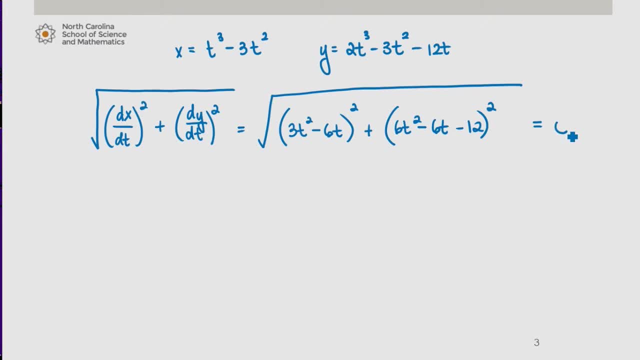 well, that can be found by answering the question: when is this expression equal to 0?? Because that means that the speed of the particle is 0.. Well, we have two expressions here that are squared, which means both are positive, and we're adding them. 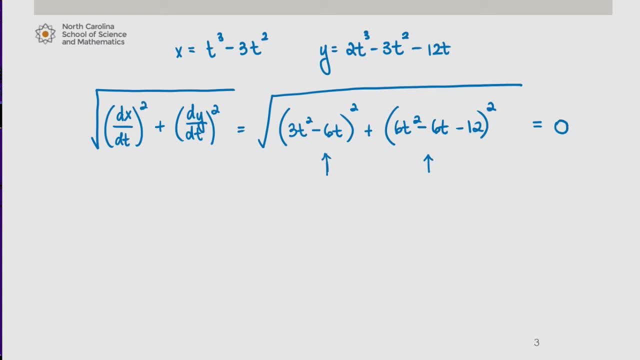 So the only way we can actually get this expression to be 0 is to identify when the radicand is 0.. Another way of looking at it is I could square both sides of this equation. Okay, Okay, Okay, Okay, Okay. 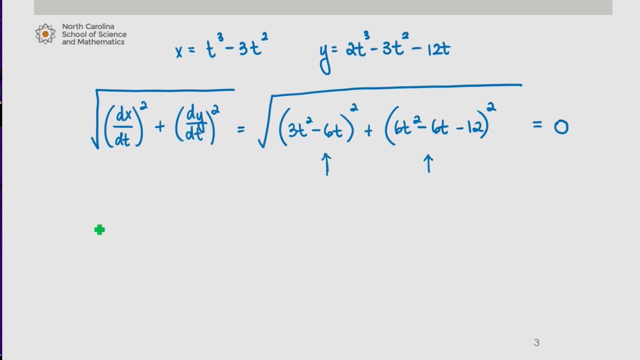 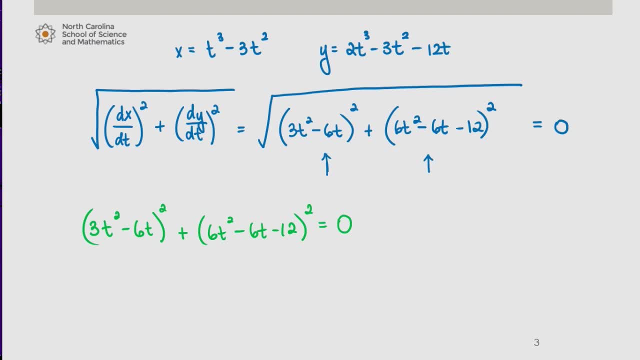 And again, since this sum is 0 and both terms are squared, neither one of these could be negative. The only way to get this sum to equal 0 is if this expression equals 0 and if this expression equals 0.. In other words, we want to find a t value such that dx, dt. 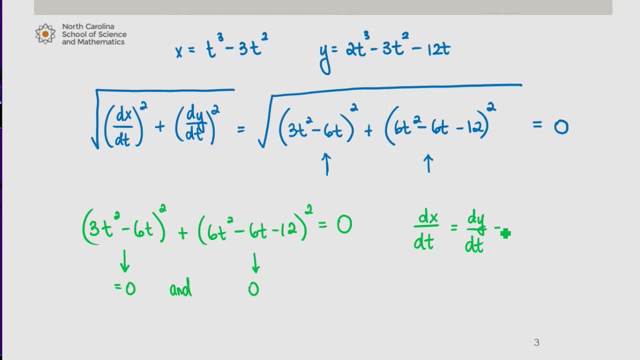 is equal to dy dt and they're both 0.. So let's first take a look at dx dt and where it's 0.. dx dt is 3t squared minus 6t. We can factor out 3t, leaving us with t minus 2.. 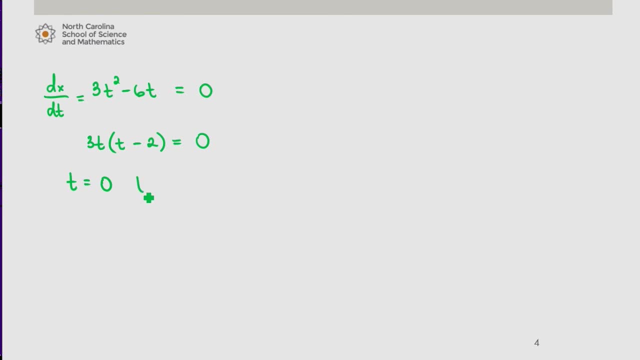 So this expression is 0. is 0 and T is 2.. dy dt, which is 6t squared minus 6t minus 12, that's equal to 0.. I'm going to factor a 6 out so I can take a look at this a little more clearly. This is T plus. 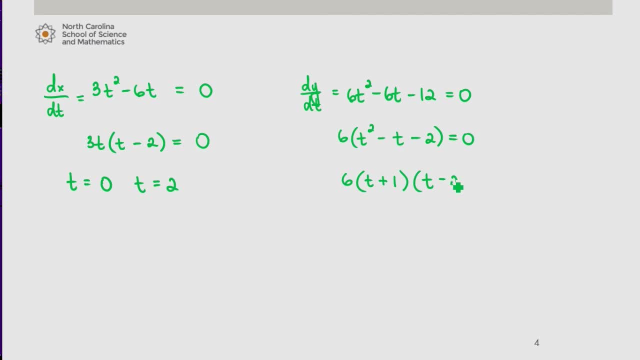 1, T minus 2.. So this expression is 0 when T equals negative 1 and T equals 2.. Now recall that we want to define when dx, dt and dy dt were both 0, so we see that happens when T equals 2.. So the particle must be at rest when T equals 2.. 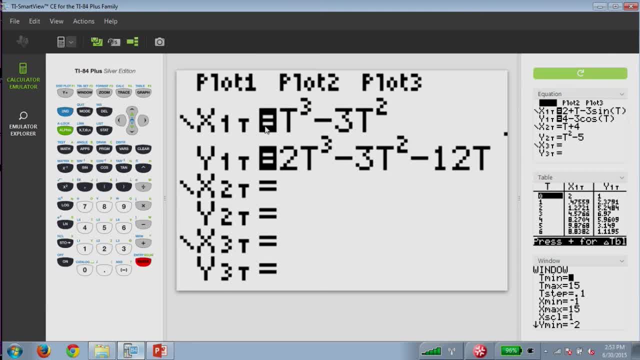 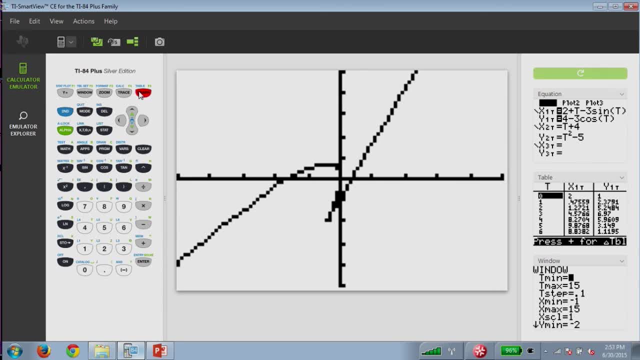 Let's confirm this by looking at the graph. So here I've entered my equations into y equals. Let me take a look at our graph. There we see, We notice that the object stopped moving at that point and then started again. Del AO.